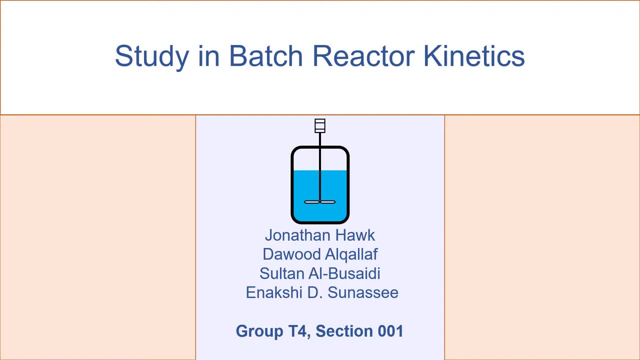 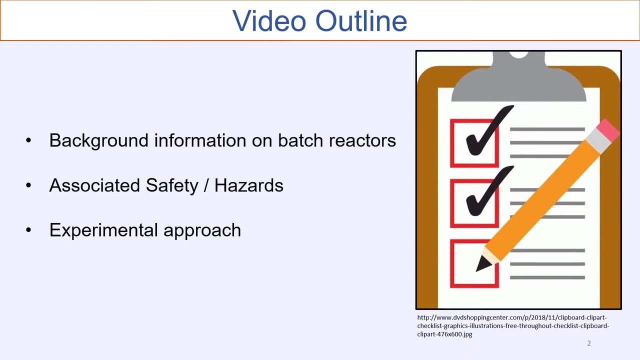 Hello and welcome to this tutorial. In this video we are going to explain the conduction of the study in bat reactor kinetics experiment as part of the chemical engineering lab. We will start with some background information on bat reactors, then discuss the potential hazards and safety precautions. 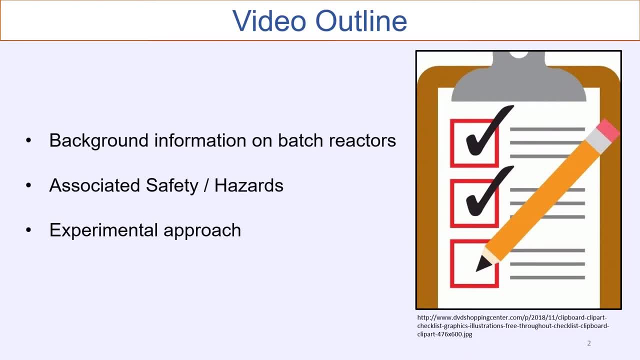 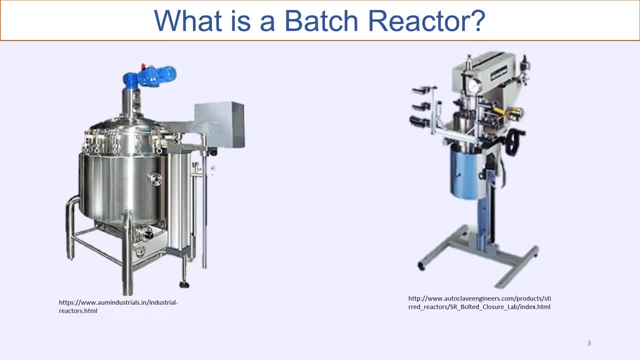 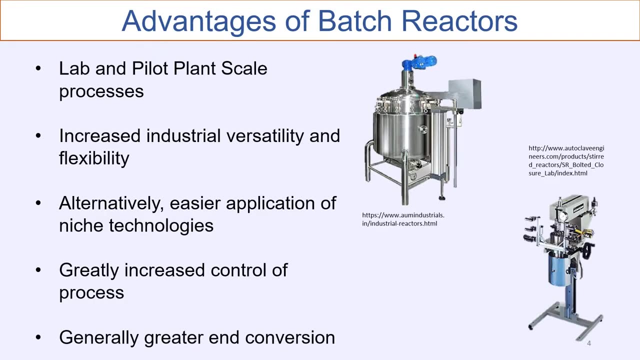 associated with the experiment and finally explain the procedure. In a bat reactor, reactants are added to the vessel initially, then the reactor is closed and the reaction is allowed to proceed. Bat reactors vary in size and operating conditions. Bat reactors are mostly used in laboratories and for 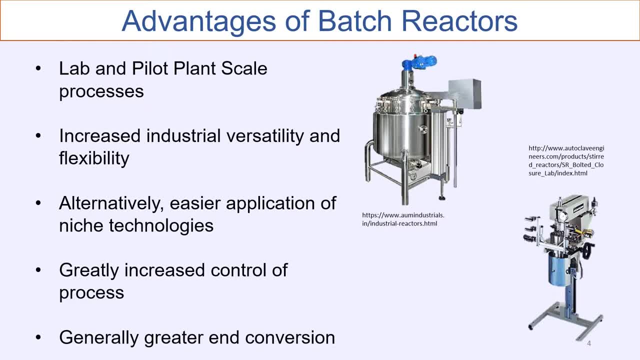 pilot plant scale processes due to their increased industrial versatility. Additionally, they allow easier application of niche technologies and greatly increased control of processes, which is important for pharmaceuticals, food or research. Bat reactors achieve higher conversions due to their increased applications, as well as increased conditionkins. Bat reactors based on your nature and adopt a high international. 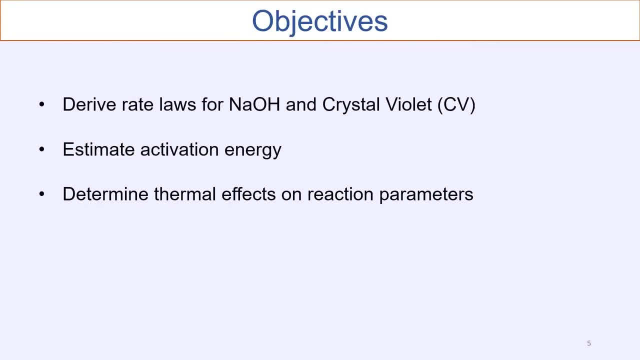 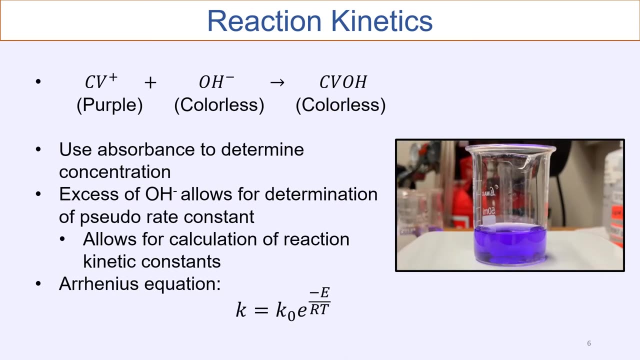 residence time. The objective of this experiment is to derive the rate laws for NaOH and crystal violet, estimate the activation energy and to study temperature effects on reaction parameters. We will consider the reaction between crystal violet, a purple solution, with NaOH, a colorless solution to form. 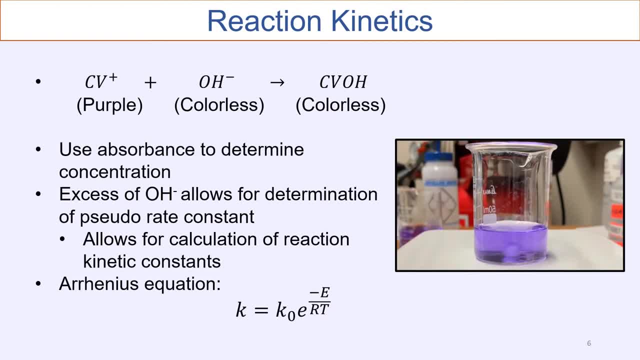 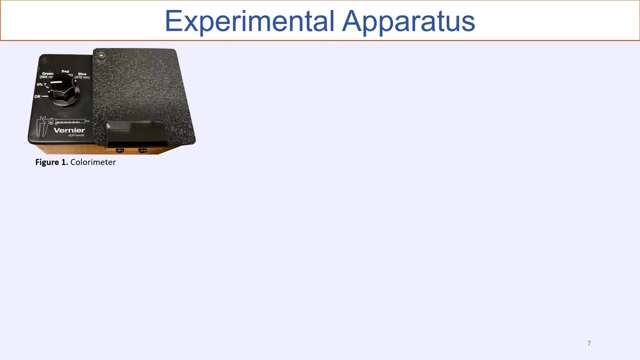 a colorless product. The absorbance of the solution is being monitored using a colorimeter. Excess NaOH was used to determine the pseudo-rate constant. The temperature is also being monitored, and Arrhenius equation is used to obtain activation energy. Let's take a look at the equipment used. We will need one. 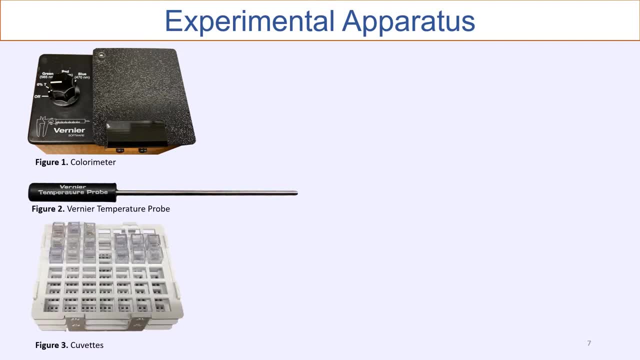 colorimeter: one temperature probe. six qubits 2 x 10 to the negative. 5 molar crystal violet solution, 0.01 molar NaOH solution, 0.02 molar NaOH solution, 0.02 molar NaOH solution and 0.01 molar NaOH solution. 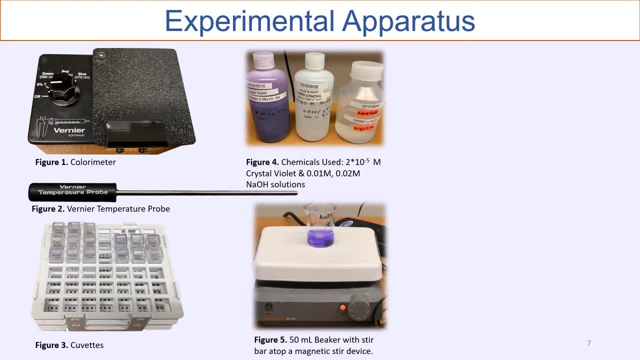 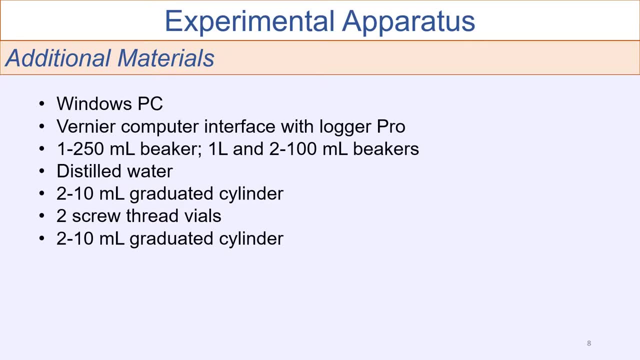 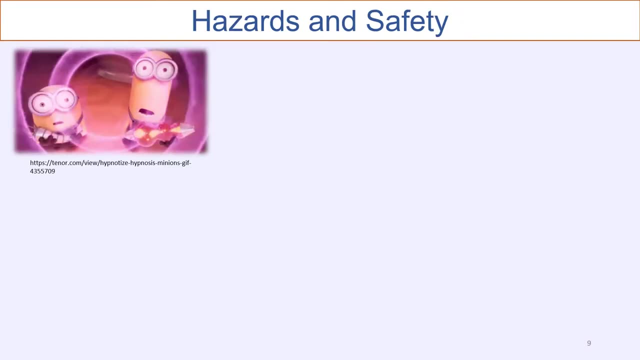 solution: a 50 mL beaker and a magnetic stirrer, variable pipette and an ice maker. Listed here are additional required materials. Now let's talk about hazards and safety When operating the colorimeter. avoid looking directly at the light beam, as it may cause. 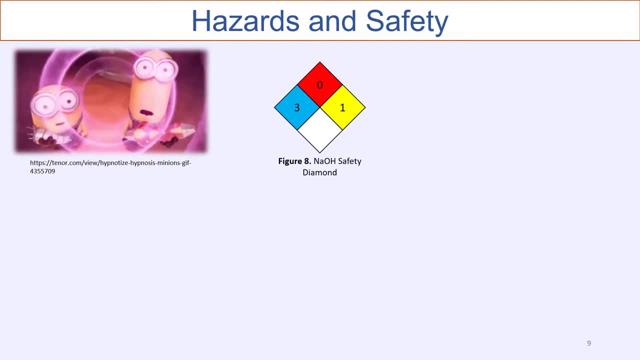 eye damage. Figure 8 shows the safety diamond of NaOH. Blue refers to the health impact, where three indicates that it can cause serious damage to eyes and skin. We are also using crystal violet, which is a biological stain, so avoid spilling it on. 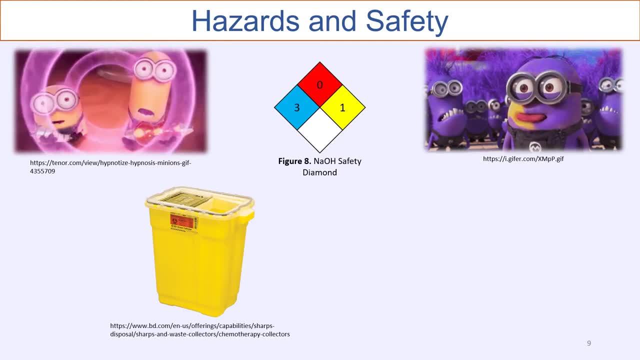 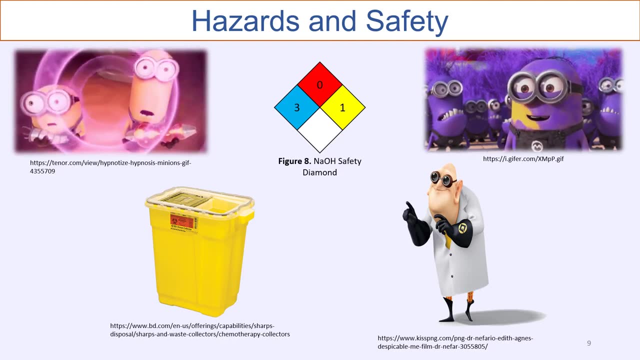 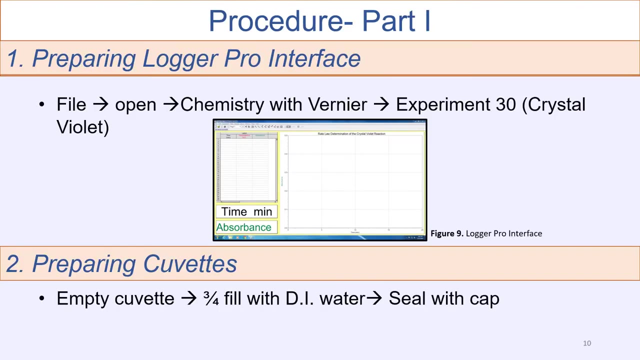 your skin and clothes. Chemical waste should be disposed off in the appropriate waste collection bins. Personal protective equipment must be worn at all time while performing this experiment, so make sure to put your goggles on, wear latex gloves and, of course, proper clothing. 5.. 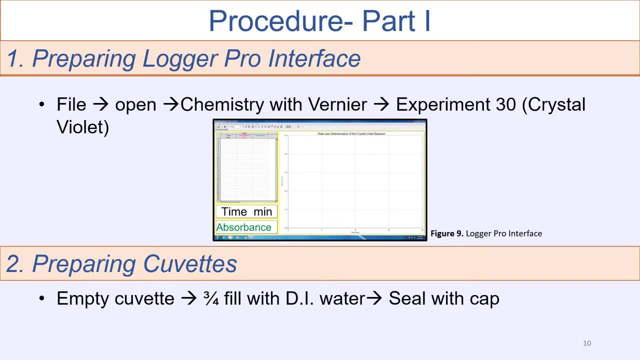 Experimental Procedure. Now let us discuss the experimental procedure. This experiment is performed in two parts. First we will determine the rate of reaction using a batch reactor, then the rate constant and the activation energy from initial rate data For the first part: first run Logger Pro. go to files. open Chemistry with Vernier. 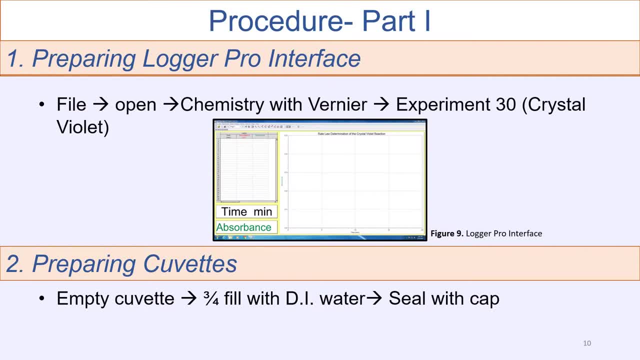 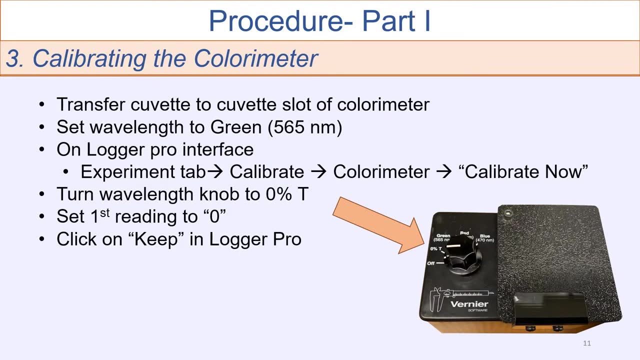 and open the file named Experiment 30,- Crystal violet. The interface is shown in Figure 9.. Clean and dry an empty cuvette, fill it ¾ with distilled water, ensure there are no bubbles and close the cuvette. Hold the cuvette by the upper ribbed edges and place it in the colorimeter. 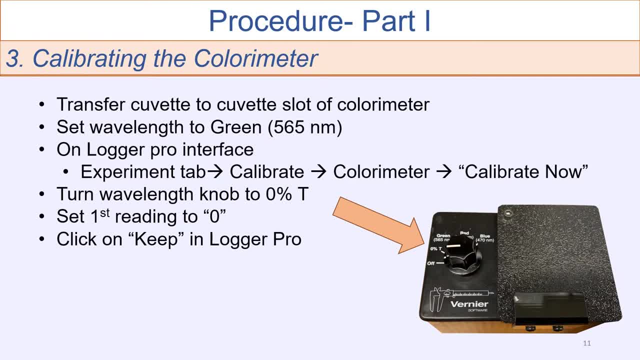 Turn the knob to green In Logger Pro. go to Experiment tab, Calibrate Colorimeter. click on Calibrate Now Turn the knob to 0% T, Input 0 for reading 1 and click on Keep when the voltage stabilizes. 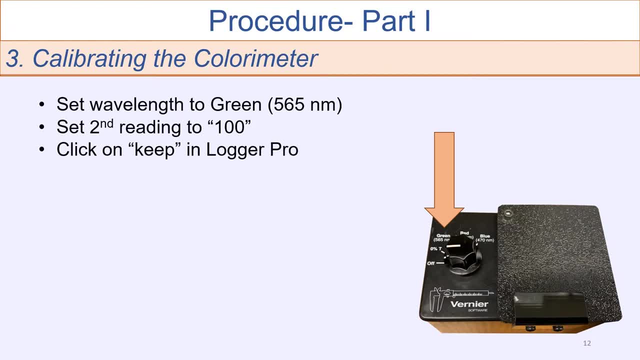 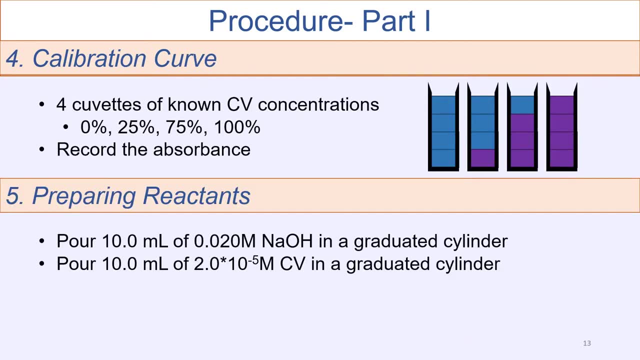 Next turn the knob to green, Input 100 for reading 2 and click on Keep when the voltage stabilizes. Then prepare 4 cuvettes of 4 different known crystal violet concentrations- 0,, 25, 75 and 100%- by volume, filled up to ¾. 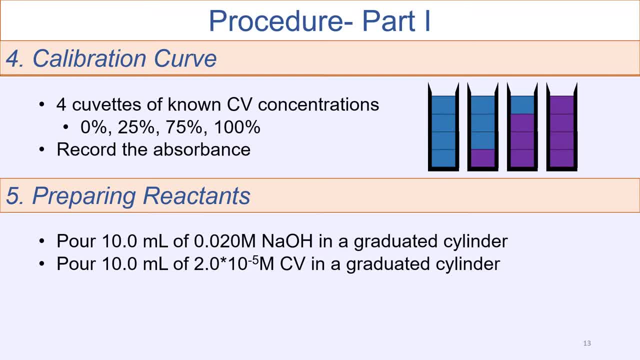 Record the absorbance of each. to finish calibration, Moving on Pour 10mL of water, Pour 10mL of 0.02 molar NaOH and 10mL of 2 x 10 to the negative 5 molar crystal violet. 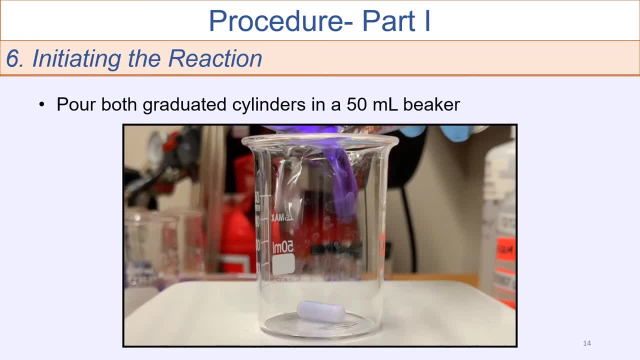 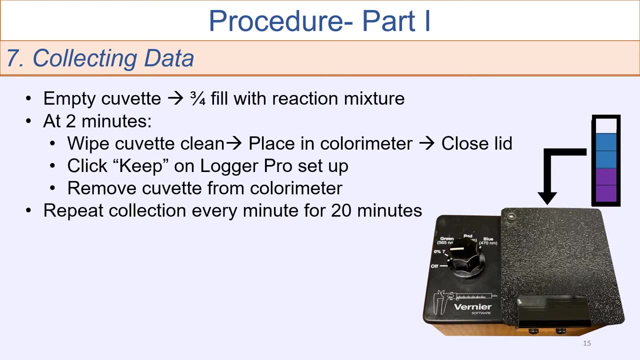 in graduated cylinders. Pour both graduated cylinder solution in a beaker at the same time. Turn on the magnetic stirrer. Fill an empty cuvette ¾ with the reaction mixture. Wait 2 minutes, then transfer to the colorimeter. after wiping and close the lid. 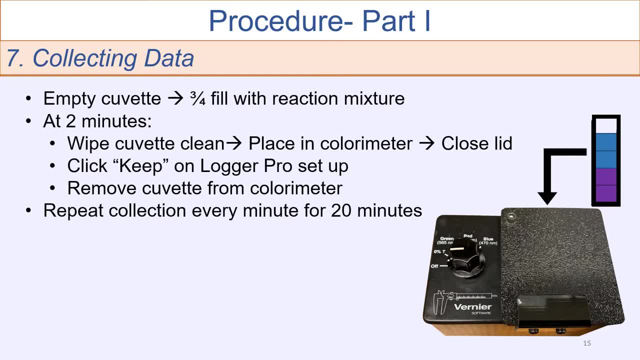 Click on Keep when the absorbance reading stabilizes. Remove the cuvette to avoid heating from the laser. Repeat data collection every minute for 20 minutes. Discard the waste in the proper disposal container. Next, repeat the same procedure using a 0.01 molar NaOH. 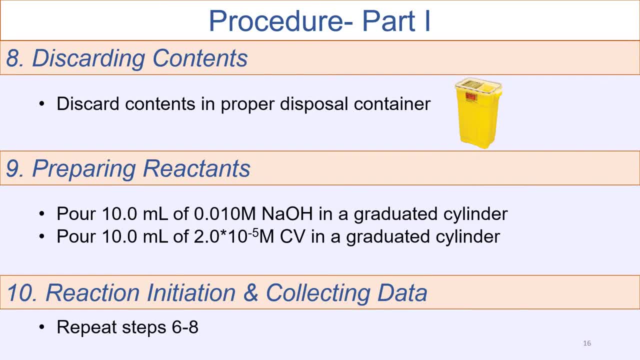 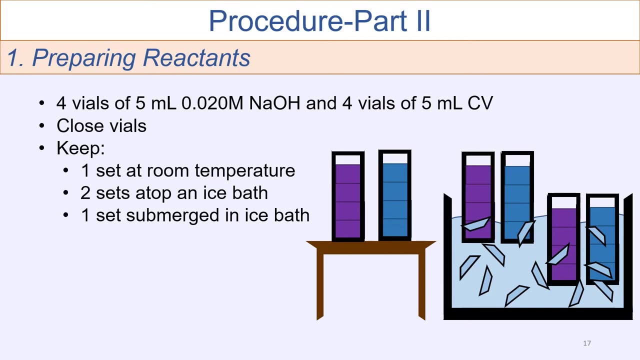 For part 2.. Prepare 4 vials of 5mL of 0.02 molar NaOH and cover the total with 0.01 molar NaOH. Pour 6mL of normal water into the container 0.02 molar NaOH and four vials of 5 milliliters crystal violet and close the. 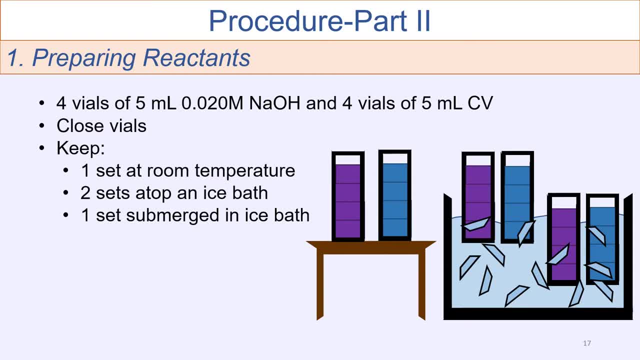 vials. Keep one set, that is, one vial of NaOH and one vial of crystal violet at room temperature, two atop an ice bath and one submerged in the ice bath. Connect the colorimeter to channel 1 and the temperature probe to channel 2.. 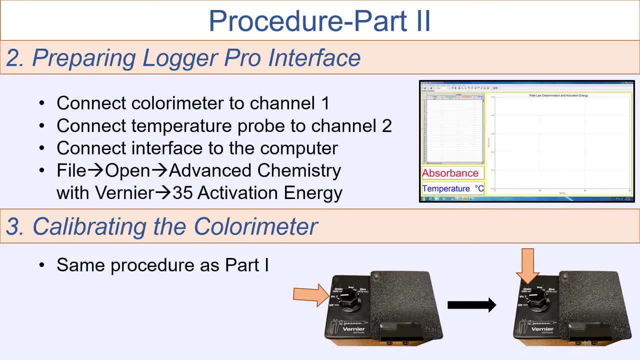 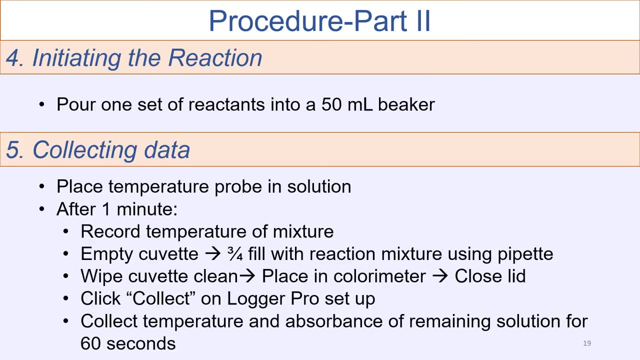 Connect the interface to the computer and run Logger Probe. Go to files, open advanced chemistry with Vernier and open the file named experiment 35: activation energy. Calibrate the colorimeter using the same procedure as in part 1. Mix one set in a 50 milliliters beaker. Place the temperature probe in the reacting. 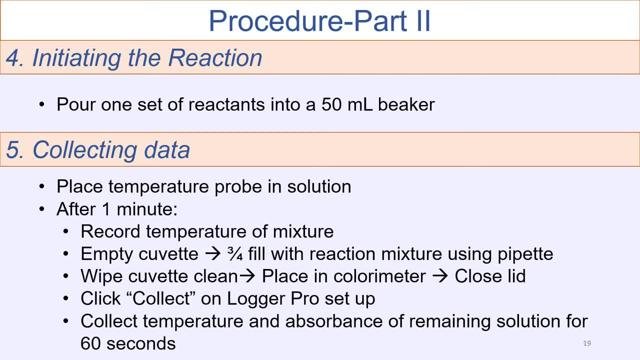 solution: After one minute record the temperature. Fill a clean cuvette 3 quarters full with the reactant Reaction mixture using a pipette. Wipe the cuvette then place it in the colorimeter and close the lid. Click collect on Logger Probe Continue to. 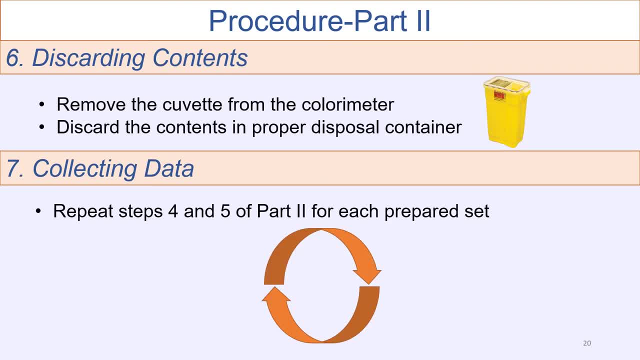 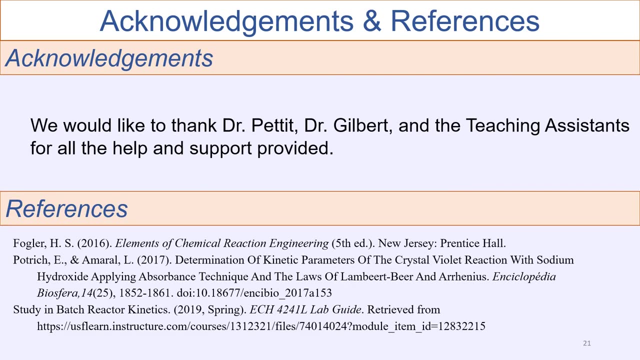 collect temperature and absorbance readings for 60 seconds, Remove the cuvette from the colorimeter and dispose of the contents in the proper disposal container. Repeat steps 4 and 5 for the remaining sample sets. We would like to thank Dr Pettit, Dr Gilbert and the TAs for all of the 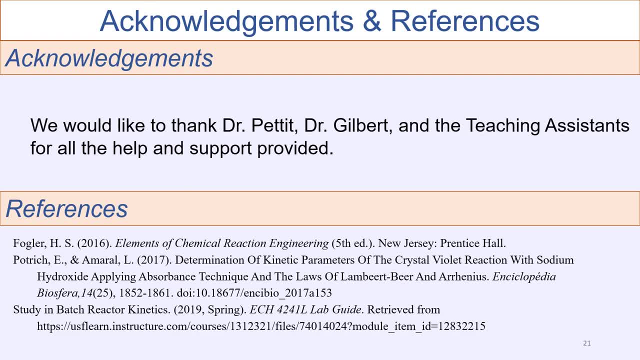 help and support provided. Thank you for watching the video.